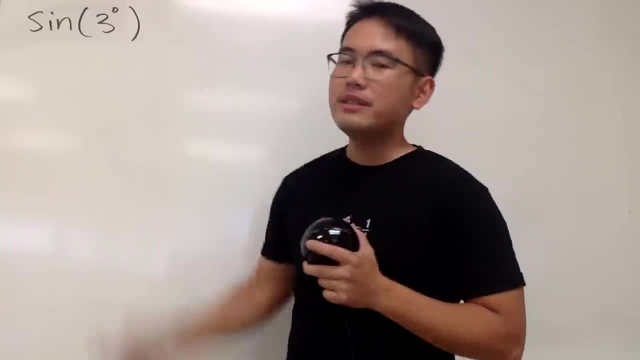 Okay, last time I showed you guys how to find the exact value for sine of 3 degrees, and it took us about 32 minutes. But today I'll show you guys how to find a really good approximation for this in under 3 minutes. 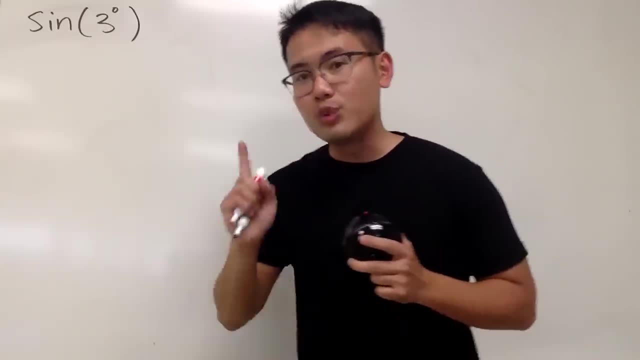 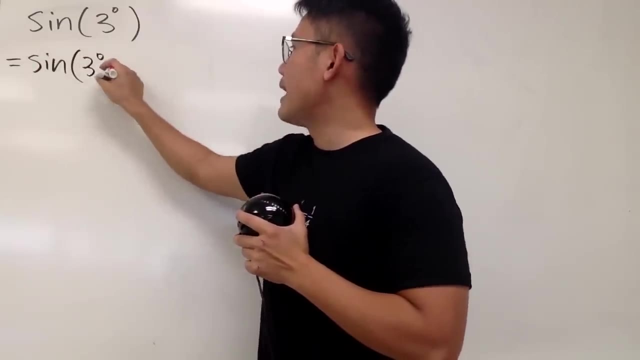 So check this out. First of all, we cannot use degrees because we are adults now, So we have to use radians. Therefore, we are going to look at this as sine and look at the 3 degrees and we multiply this by pi- over 180 degrees. 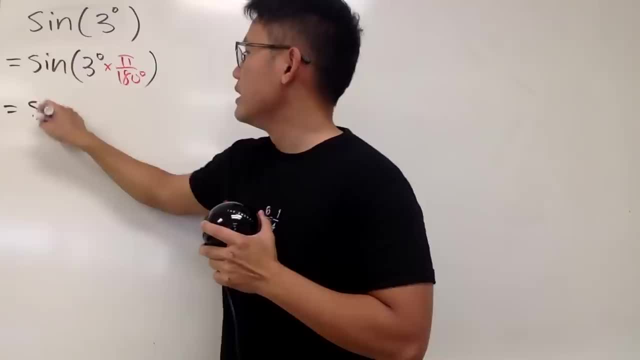 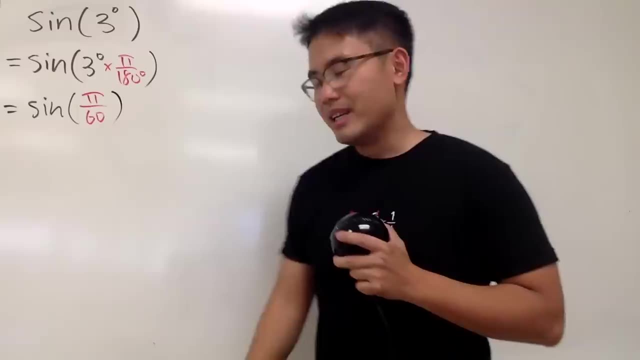 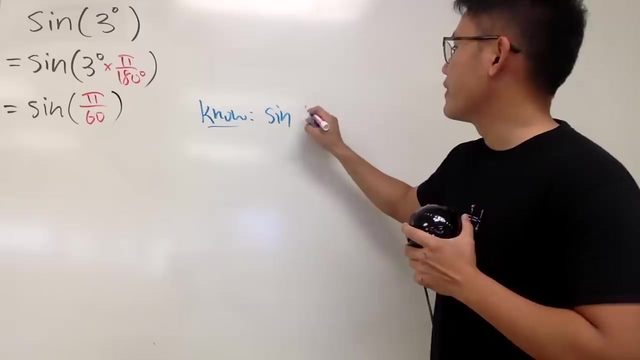 And of course we can just work out the inside, and this is going to give us sine of work this out. you get pi over 60.. And now we are in business because we can use the Taylor series right here. As we all know, whenever we have sine of some angle theta and let's say we are just doing the Taylor expansion center, DSU row. 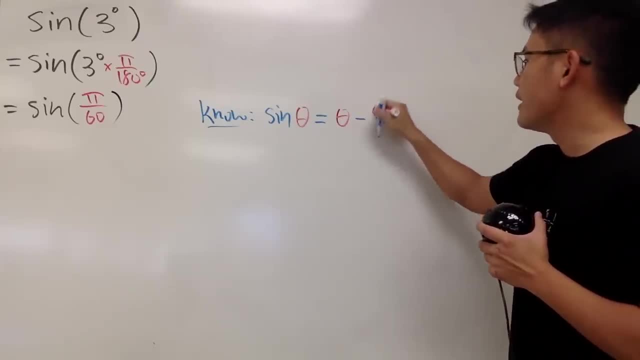 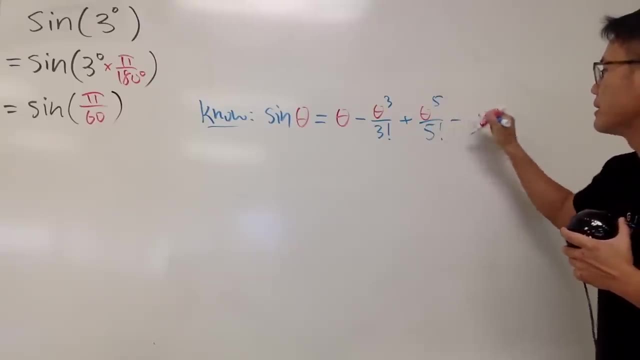 we have theta here and we minus theta to the third power over 3 factorial and we add Theta to the fifth power over 5 factorial and then subtract, and so on, so on, so on. So this is the Taylor series. expansion for sine center- DSU row. 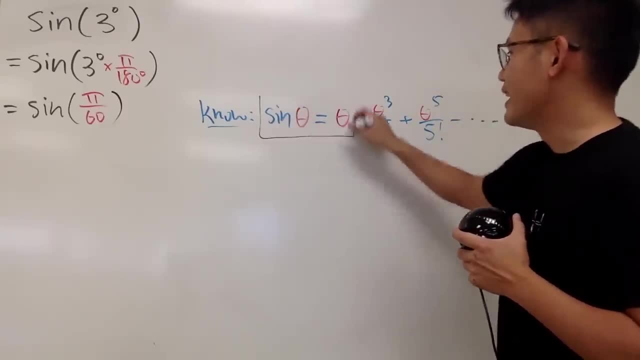 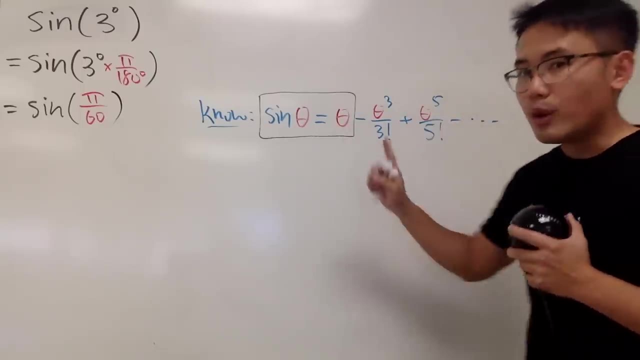 The key words: center DSU row And if you are willing to just take the first term, Whoa. As we can see, we have sine. theta is equal to theta. However, we have other things after that right, So this is no longer an equation. 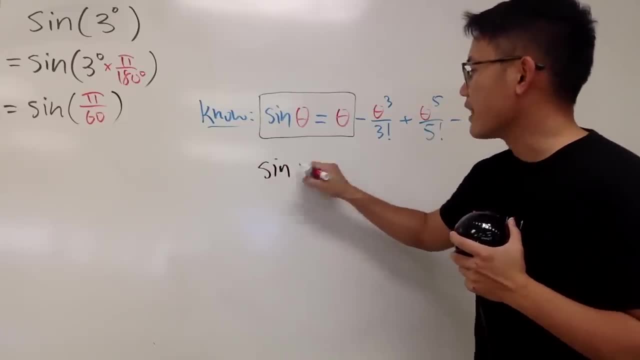 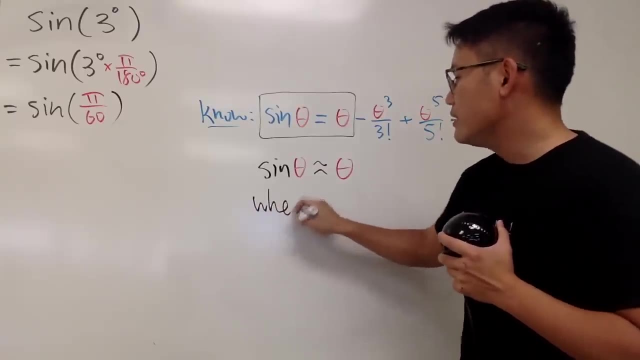 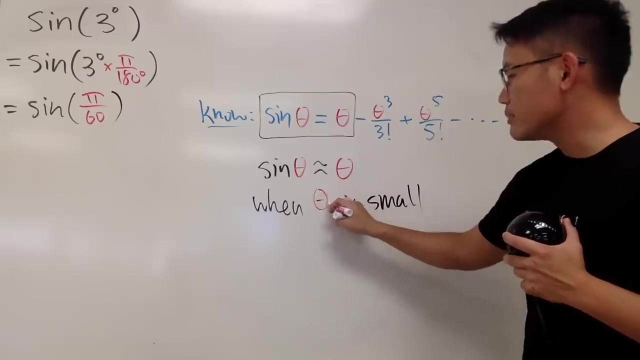 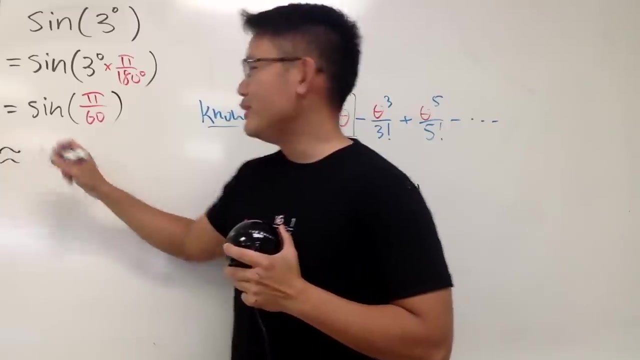 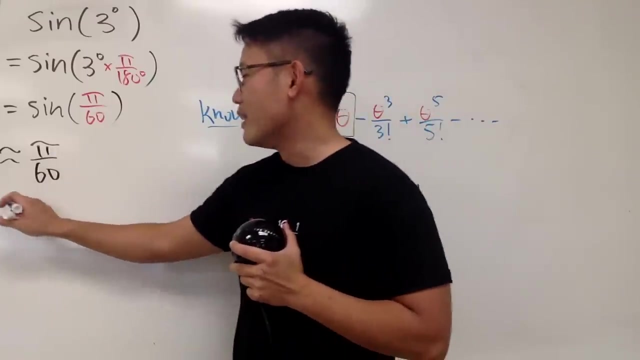 This is just going to be an approximation, So we can write sine. theta is approximately equal to just theta, But you do have to attach. So this is the, And of course you can just use the calculator right here. If you do the approximation here, you get 0.052359 dot, dot, dot. 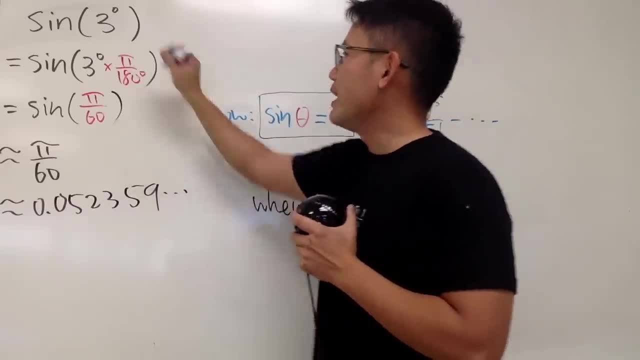 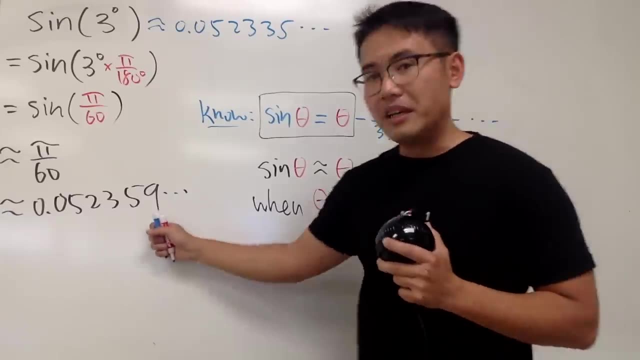 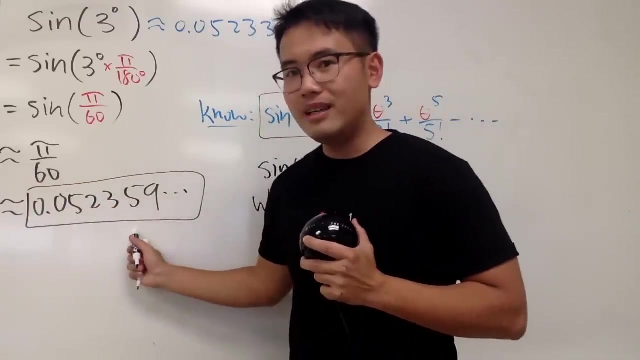 And if you use the calculator to do this right here, you get approximately 0.052335 dot dot dot. As you can see, this is pretty good right. Therefore, there you have it. This right here is the approximation answer for that. 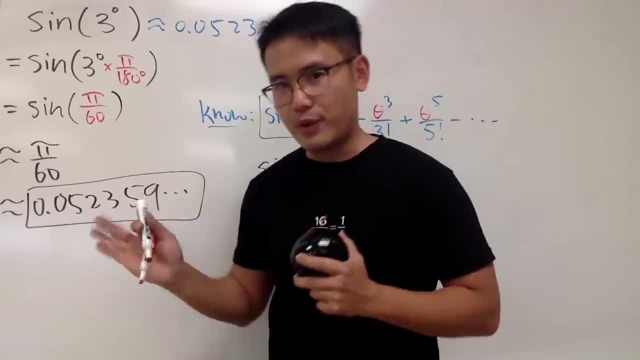 You know what I can't even. This is genius. Very cool, Under three minutes, as I said. Thank you guys so much for watching.